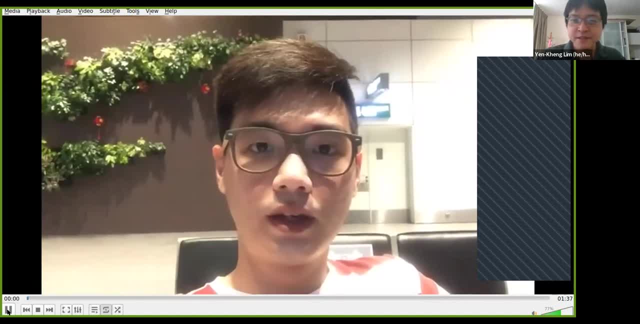 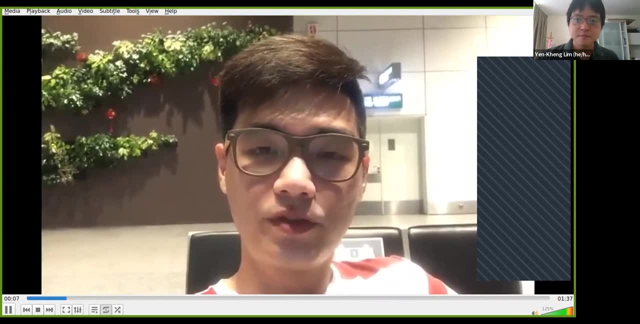 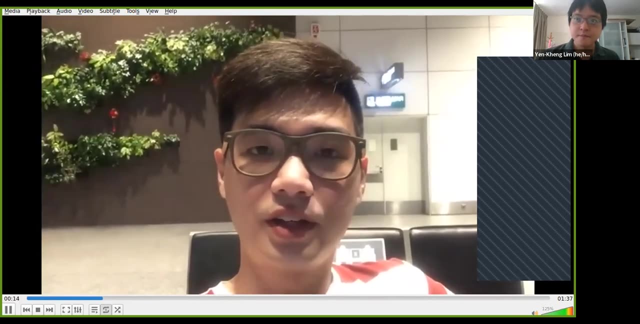 but let me play his message to everyone. President of the Logic Association of Malaysia. I am currently waiting for my flight to New York from Kuala Lumpur, And so at the time of the first session, I will be on the flight to New York And 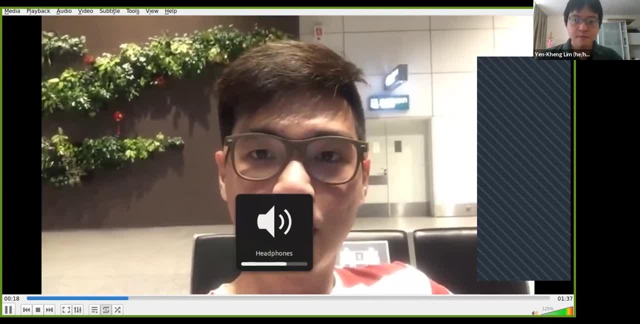 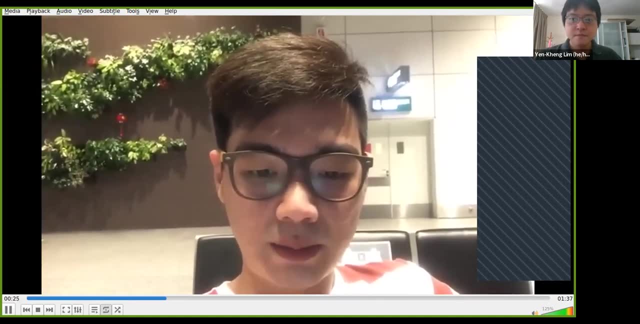 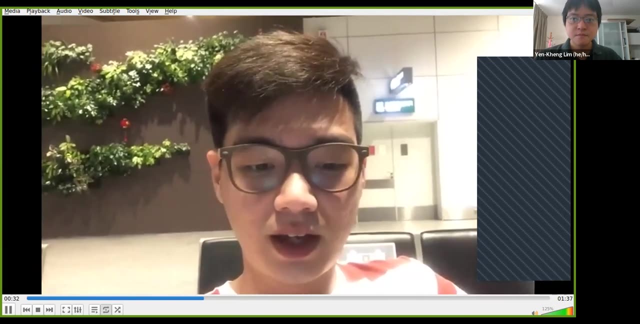 so I have to do this recording to give you a quick forward. Yeah, so I would like to welcome you to the online annual introductory logic course series aimed at giving young aspiring mathematics, philosophy and other science students and opportunity to get to know what mathematical logic is like and to decide if he or she wants to pursue it further after taking the course. 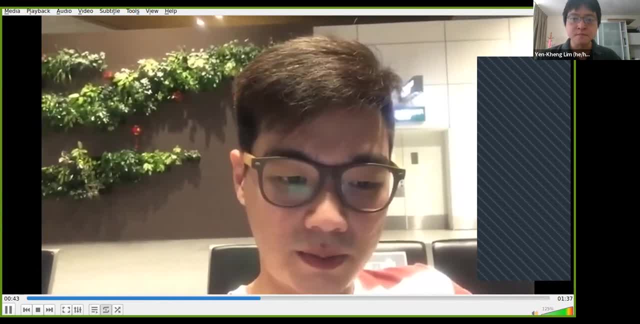 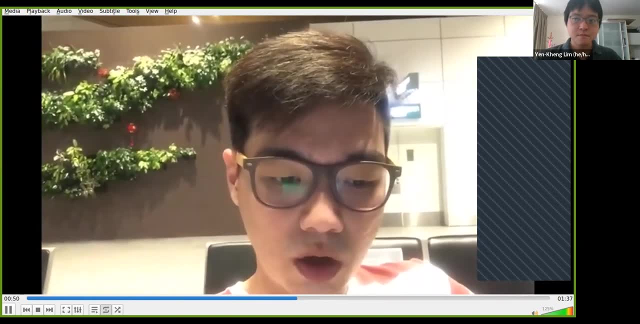 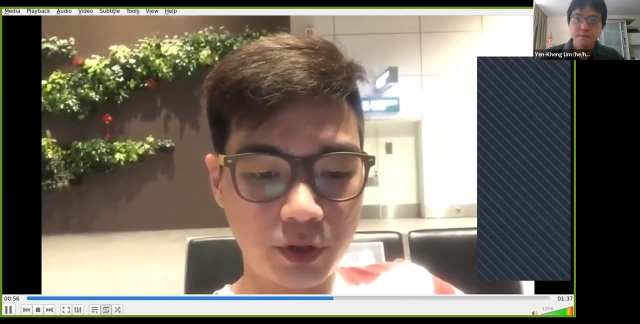 We are delighted to have five excellent instructors to conduct the course. We have Athipat Tamrung Phanyalak, Diana Bartisova, Jiachen Yuan Jun Le Goh and Patrick Lutz. We also want to thank our sponsors of the program Nu-Plus Manufacturing ArdenEDU and our sponsor, New Plus Manufacturing ArdenEDU. 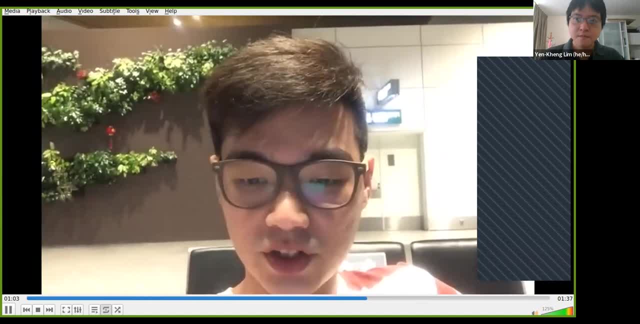 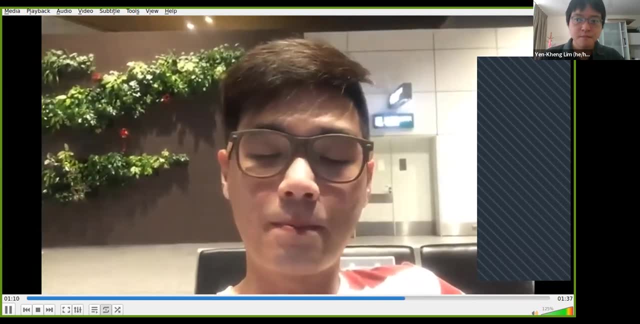 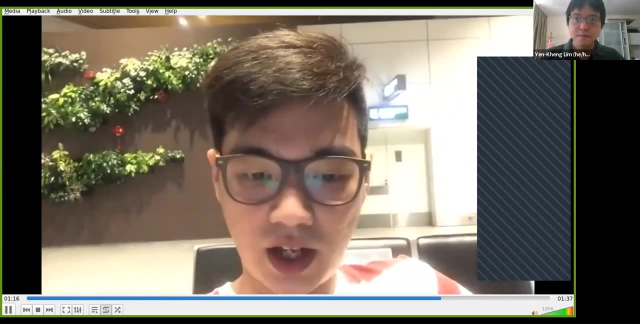 and more. Do spend time exploring the services they provide and offer, and perhaps I can give you a discount if you mentioned that you were a participant of this program. Also, a special thanks to Professor Koji Nakatogawa of Hokkaido University for his kind endorsement of the program. 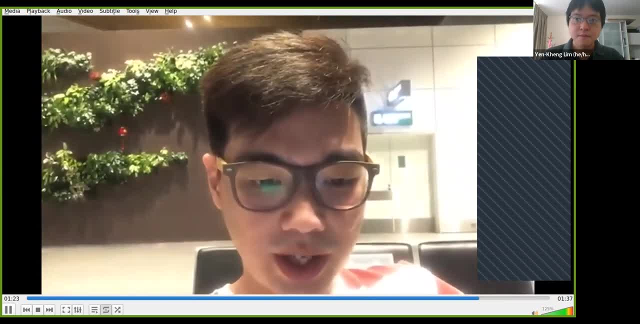 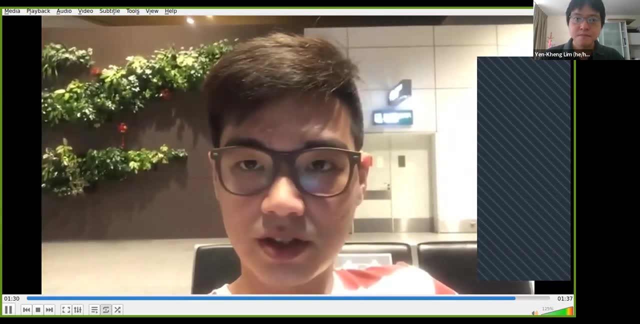 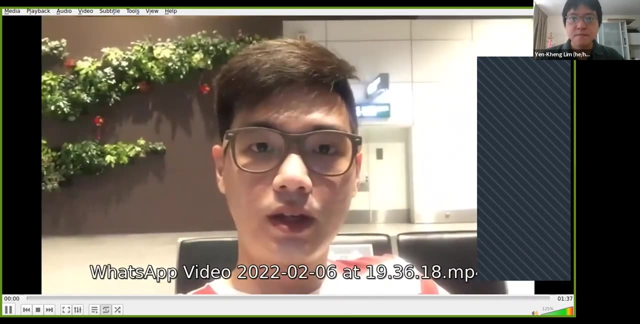 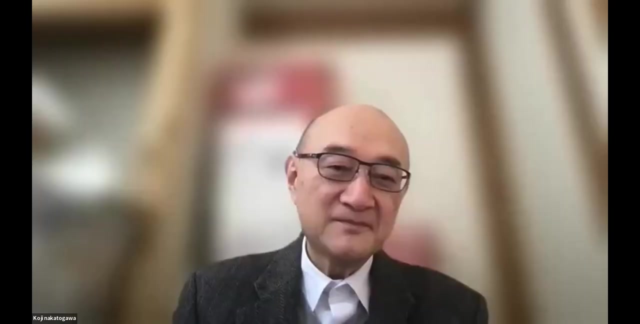 Thank you, Professor Koji Nakatogawa. I hope you will enjoy and profit from this course, as all of you do visit the website often for notices and updates. With that welcome and see you again, I mean see you, Hi. Okay, so that was Tzu-Yao. I think we can begin for today's. 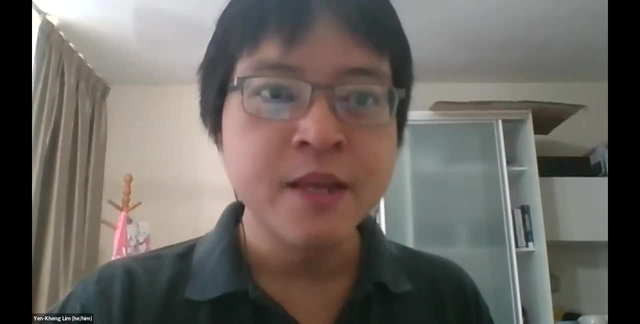 session. Let me introduce the speaker for today. Today's speaker is Dr Atipat Tamra. He's from Chulalongkorn University, Thailand, and he got his PhD from UCLA under the supervision of Matthias Aschenbrenner, and his PhD title is Extensions and Smooth Approximation of 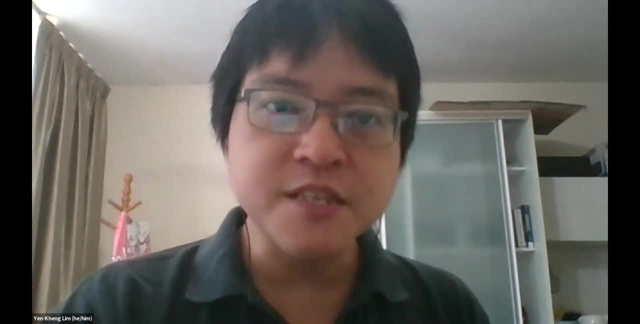 Definable Functions on O-minimal Structures and his research interest is on model theory. So his series of lectures will be about first-order logic introduction and the model theory portions. So he's going to be talking about the first-order logic introduction and the model theory portions. 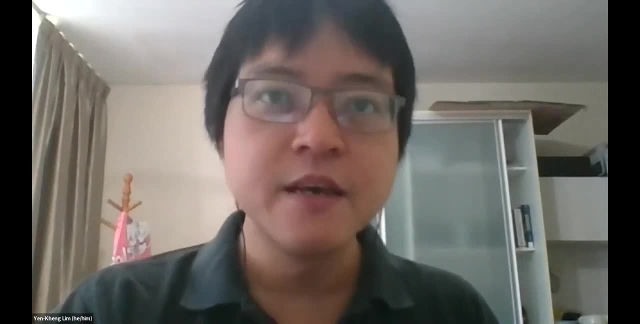 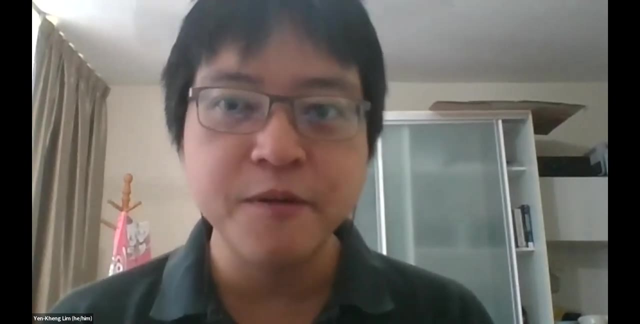 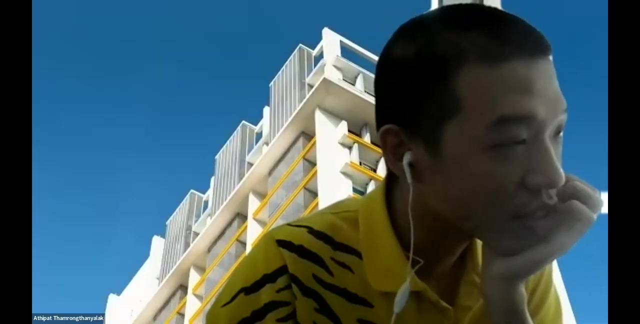 This part for the course is these topics. So, without further ado, I think I can pass over to Dr Atipat. You can begin your presentation, So you can go ahead and share your screen. I think Okay. Thank you for the introduction. Could you please enable me to share my screen? 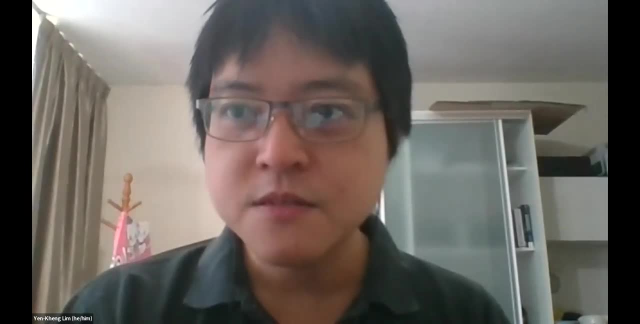 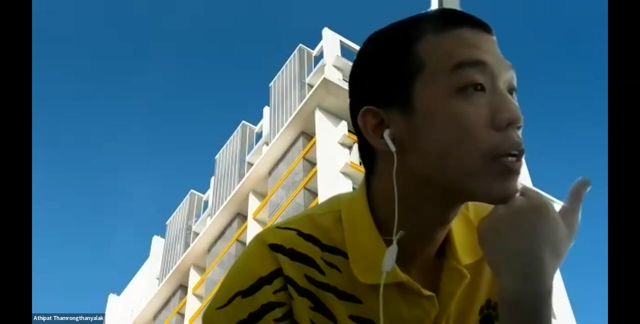 It's disabled right now. Hang on, Yeah, So So I'm not entirely. can I make you the host, or You can make me, or you can make me co-host? I think that should give me permission to share my screen. 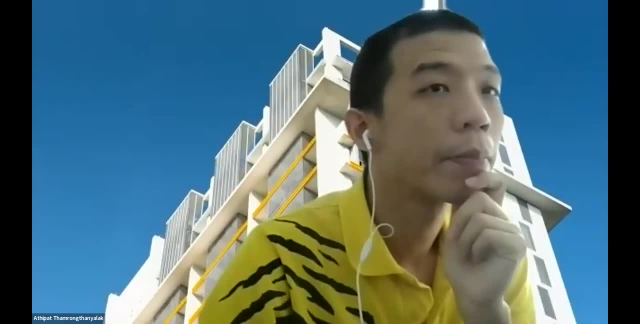 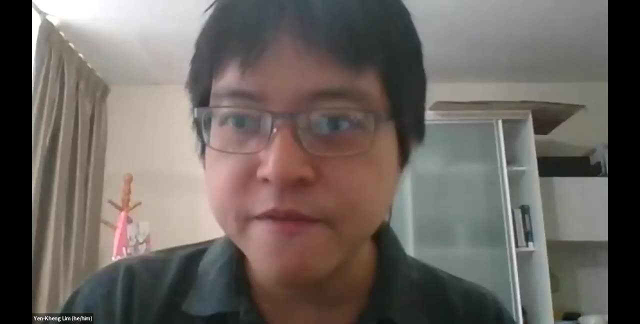 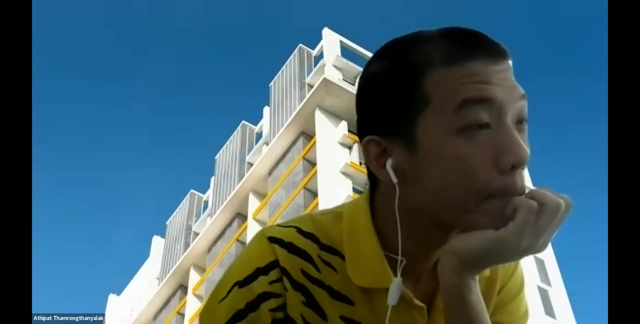 You can right click on my name, I think, and click make co-host. There's no option for co-host? Oh, there's no option for co-host. I think we can allow them to. Oh, yeah, yeah, yeah, You can do that. 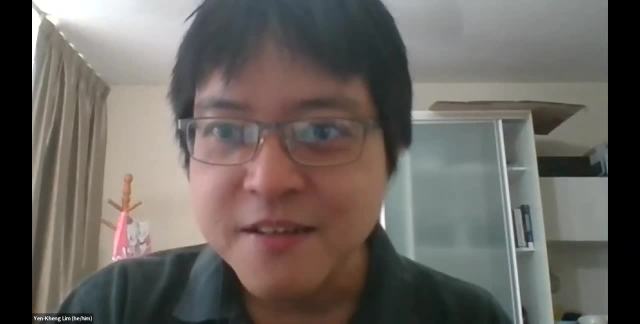 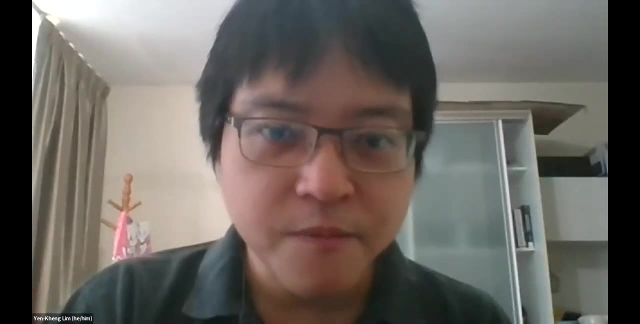 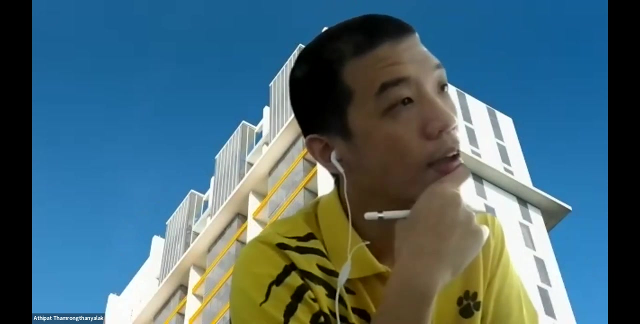 Yeah, I need to remember how to find it. I think you can just setting. Are you using PC? Yeah, I'm on the PC right now. I think you can click the up arrow button on the share screen button. Yeah, I think they should have some option there. 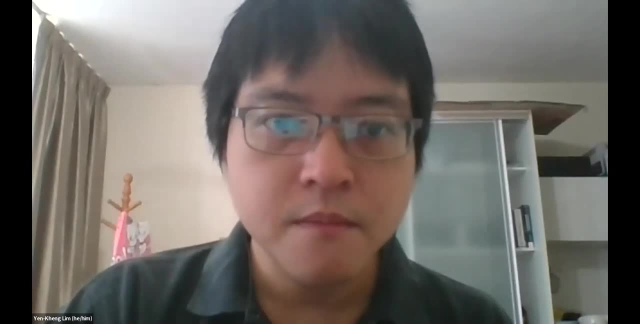 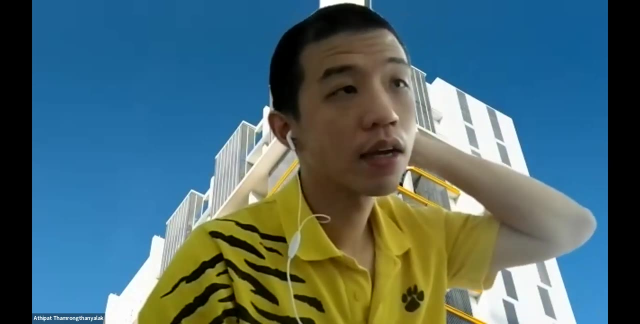 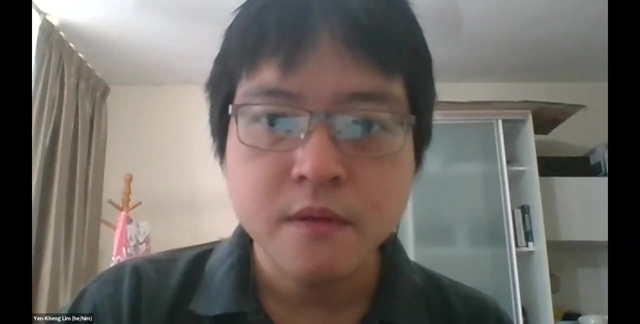 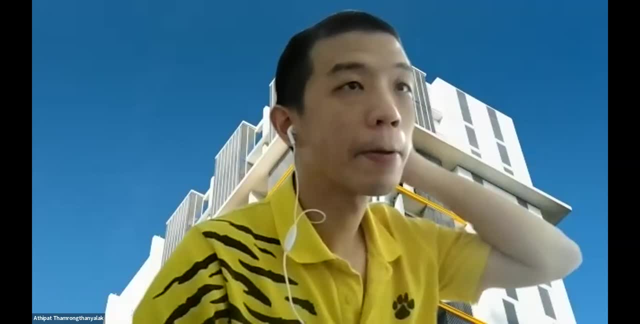 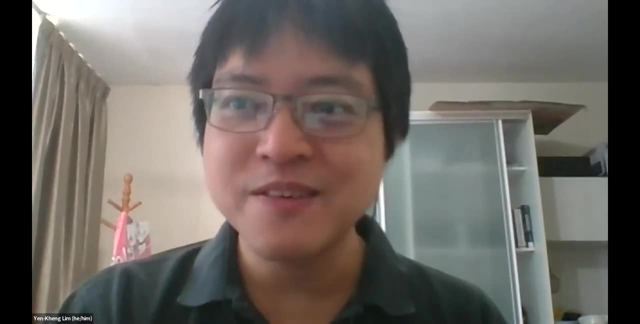 Oh, okay. Yeah, apologies to everyone. Yeah, apologies to everyone. So I think you're in charge, So I think you can share the screen now. Okay, Actually, I changed the setting for you. Let's try that again. 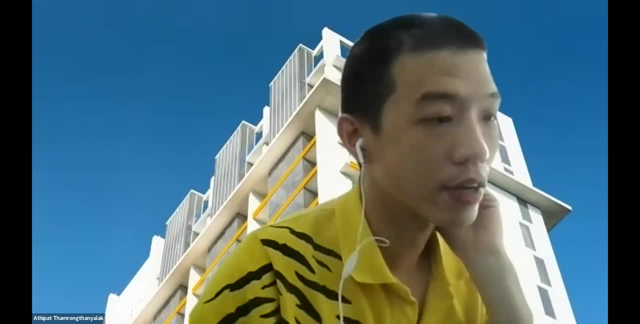 Oh, okay, you Let's try. I can say: